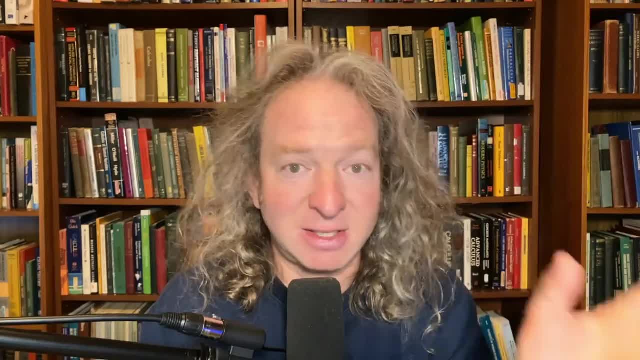 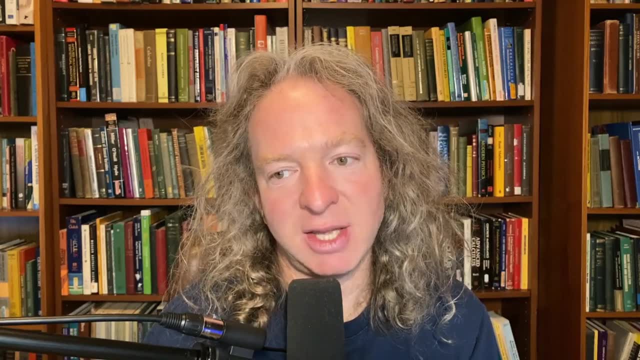 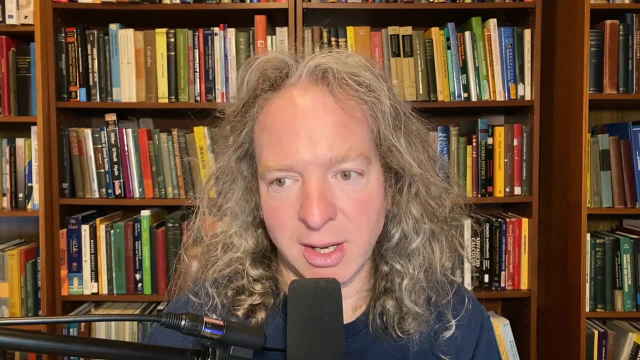 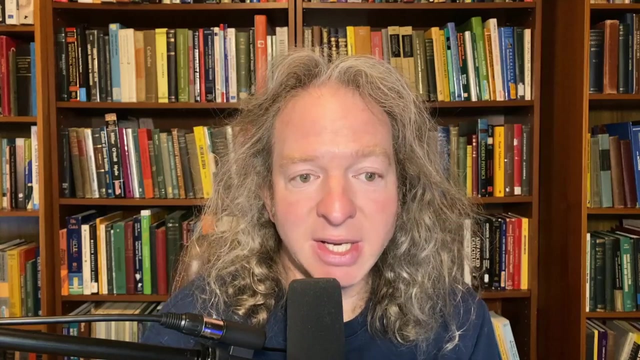 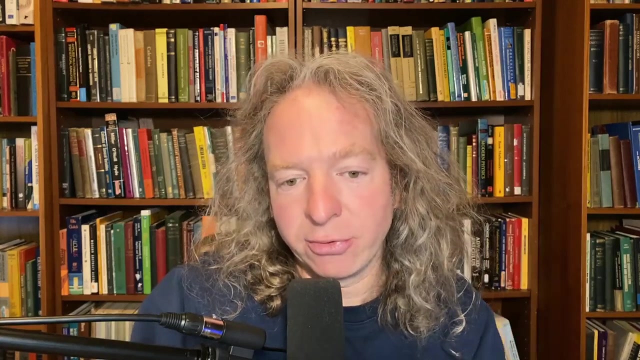 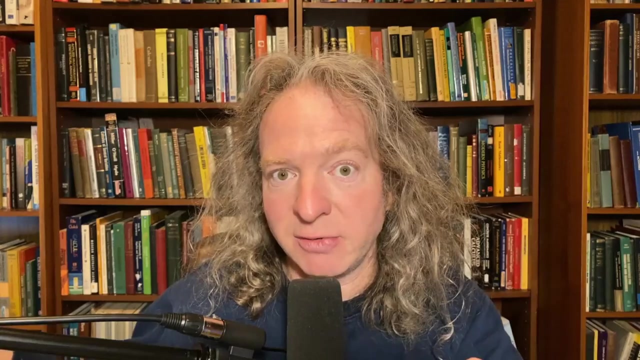 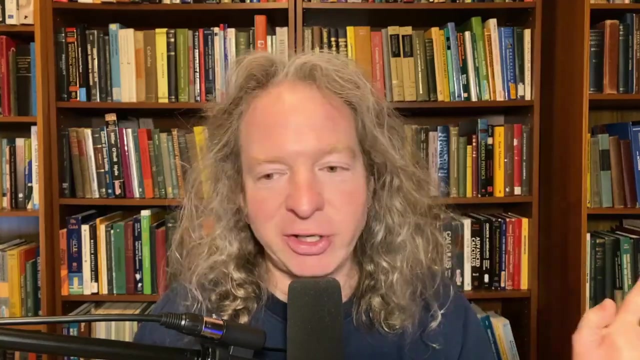 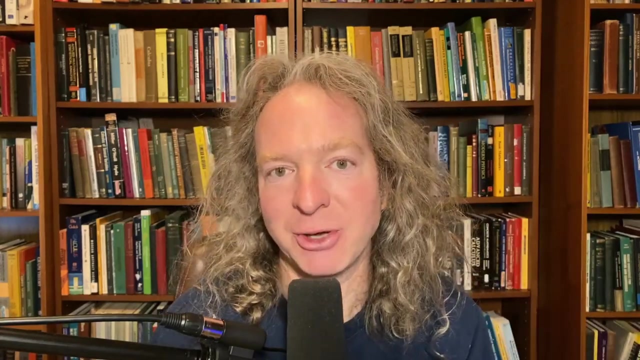 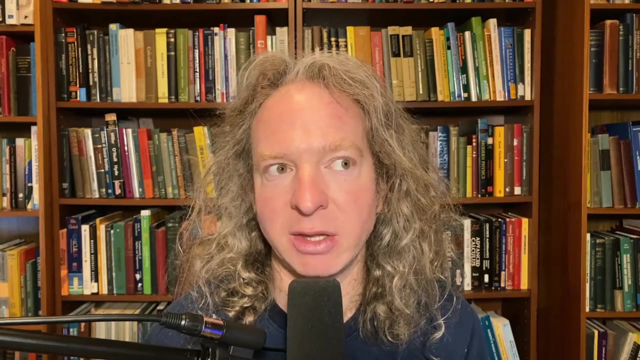 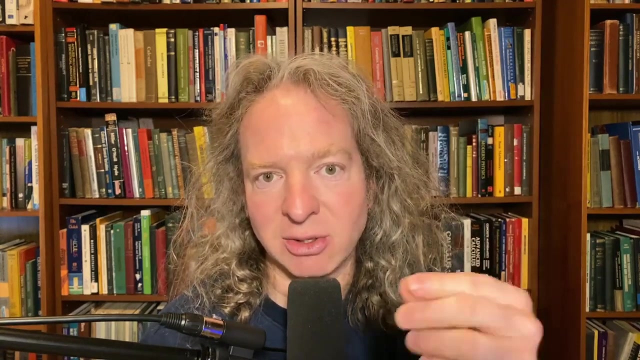 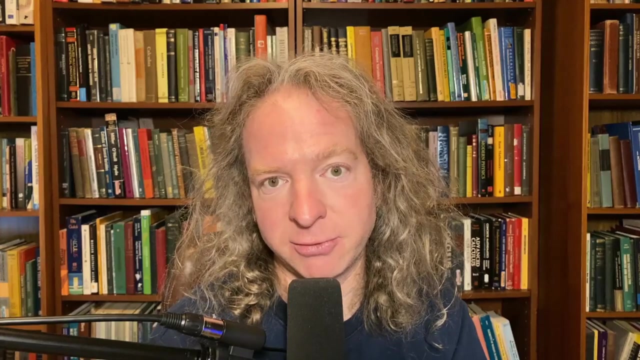 say an undergraduate math degree or you know and some of the grad school stuff that's a lot of math and that's what was covered in that video uh yeah don't be intimidated it is a lot but you got to remember that you know i studied mathematics for a very long time right very long time i was in school uh for a long time i took a lot of math classes so yeah you know it takes years it takes years so my advice is to get a book so number one get a book on writing proofs if you get a book on proof writing what that's going to do is it's going to open the door for more interesting advanced mathematics which i'm going to show you later in this video so as far as getting a book on proof writing there's all kinds of books i have several i was looking for one and i know i have it and i can't find it but i couldn't find it it's the book by velman okay the book by velman how to prove it i think that's a really good one i don't know if you can access that book in croatia i was trying to think before making this video when i read your email before making the video thinking what book can i recommend that you can access in croatia and i just thought of one right now there's a book online it's called book of proof it's free it's 100 free you can buy it from amazon 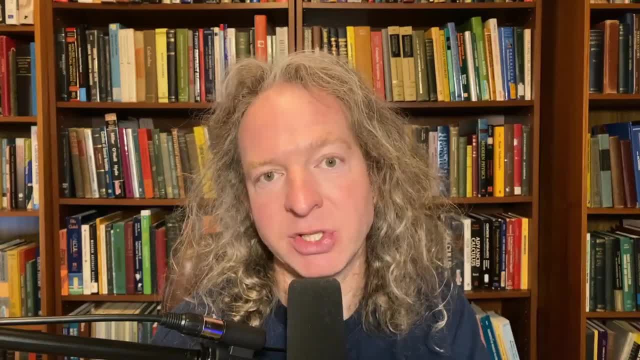 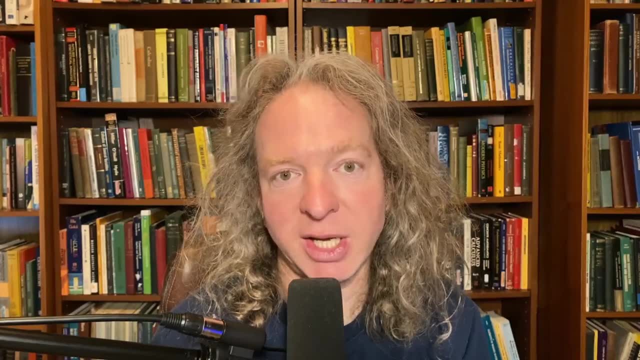 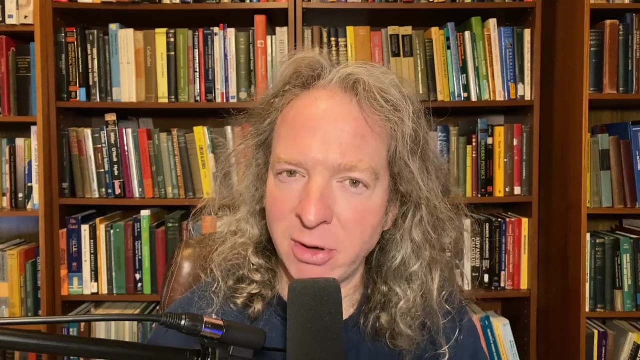 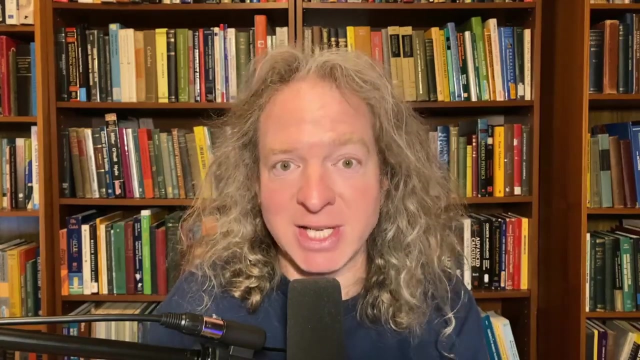 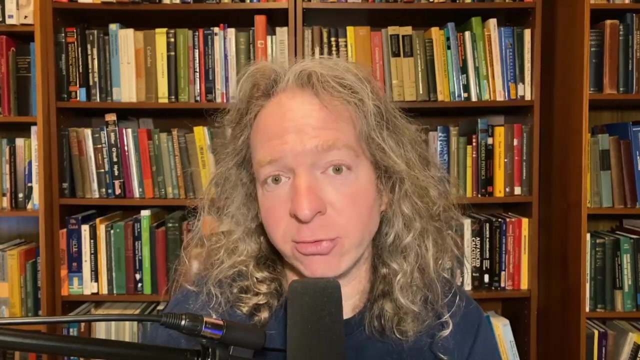 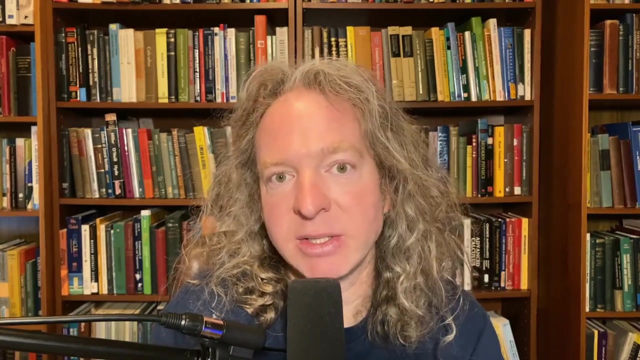 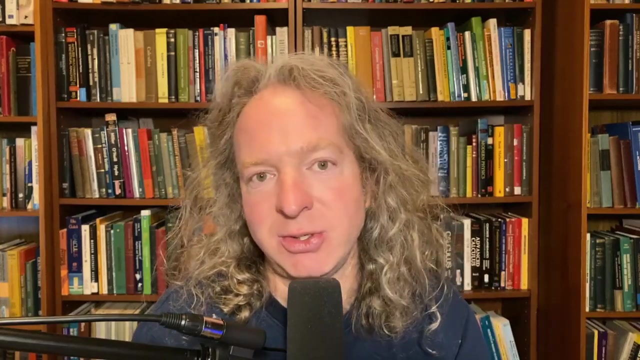 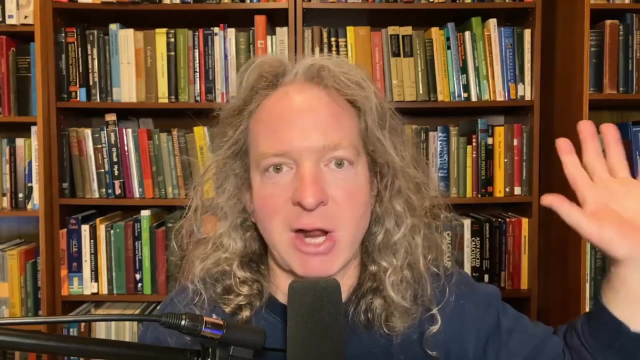 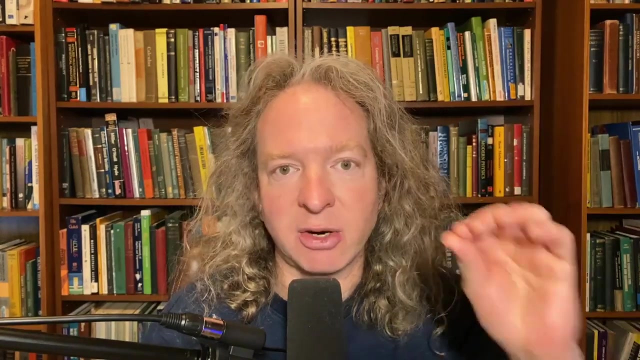 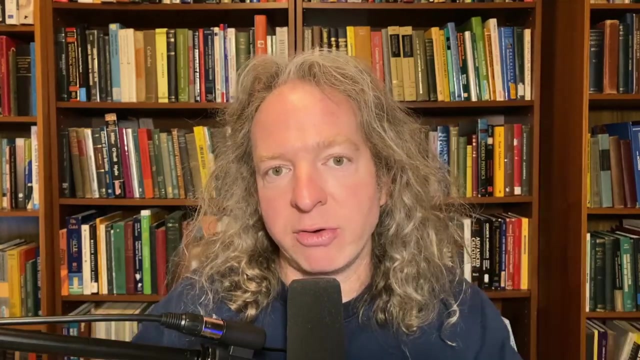 i actually bought it i have a physical copy in paperback that i purchased on amazon but the book is free it's written by richard hammock it's called book of proof so that's a free version that you can get it's pretty good i've done maybe 20 episodes of book of proofs in croatia exercises from the book and i've looked at maybe 80 percent of the book i've glanced over it and i've maybe read one or two chapters fully that's my experience with the book which is pretty good i've looked at almost the entire book i've looked at solutions you know i've i've looked at it a couple times i made a video reviewing it it's called book of proof and what you want to do with that book okay is you want to sit down every day and you want to work on it for like 30 minutes okay and that's how you really take it to the next level because that's like you know that's not passive that's not just like watching a youtube video or you know watching you know another youtube channel which is mind your decisions which is a really famous channel it's been out for a long time i think he does like tricky math problems you know those are great those are great youtube it's a great youtube channel it's got great videos but like you're not going to get really good unless you sit down with a book like book of proof and work through it so that's one option another option is the book by velman okay again i think that's i think that's 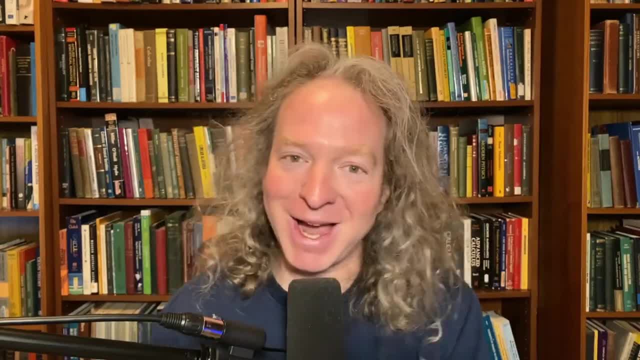 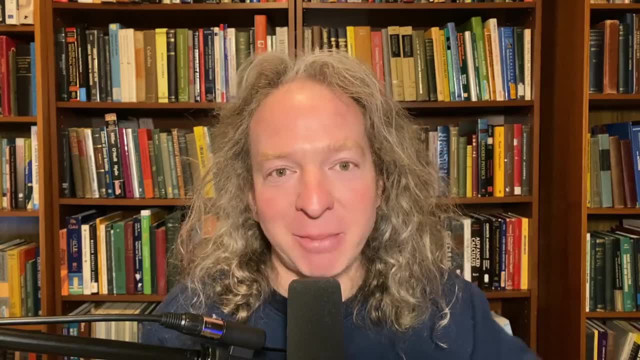 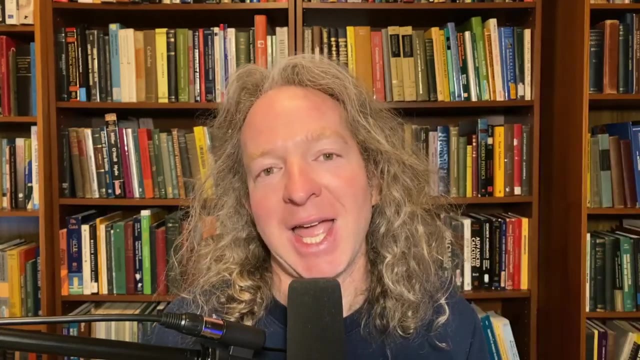 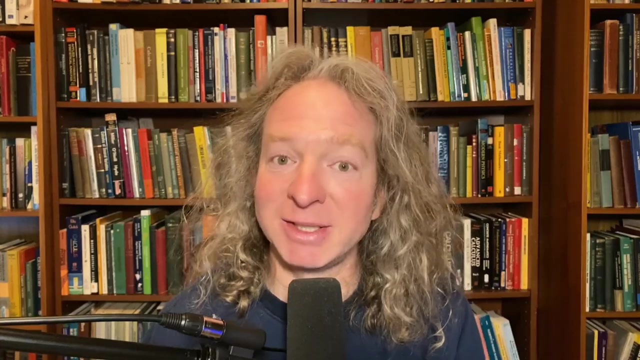 portable i grudgingly bought that book i i did not want to buy it uh i feel like i feel like i was pressured to buy it people kept leaving um comments about that book a few several months ago maybe a year ago and they're like oh you got to check out the book by velman because i was talking about these other proof books then and i bought it i'm like oh what i want this book and i started reading it like oh i already know all this stuff it's kind of boring and then i forced myself to read it and i'm like this is pretty good it's got a lot of stuff in there and 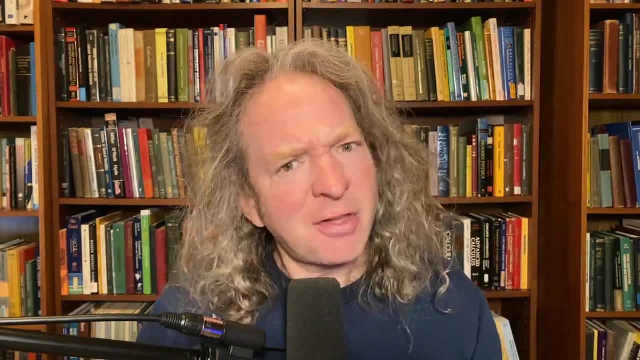 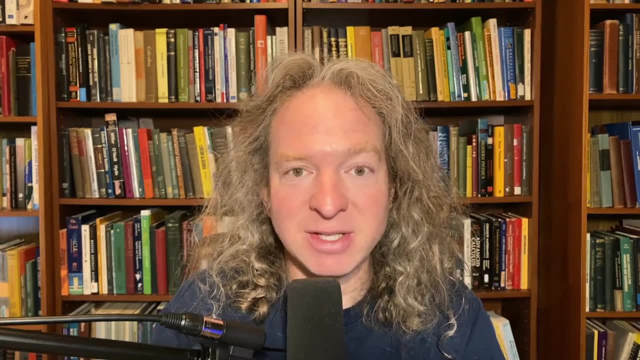 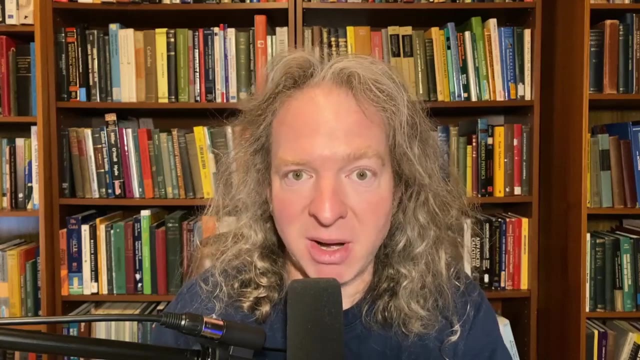 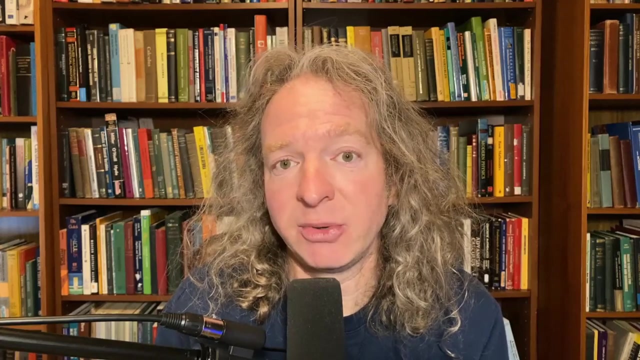 his take on different things like he talks about vacuous truths i thought that was really enlightening and i thought that velman did a good job so the book by velman is phenomenal um i don't want to say it's my favorite proof writing book but it's definitely the one i'm recommending to you um i also like the book by bond and keen it's also a good book again bond and keen but the book is good and in croatia you'll definitely be able to get book of proof because it's free so it's available to anyone in the world thanks to the internet again just google book of proof richard hammock and you got it okay 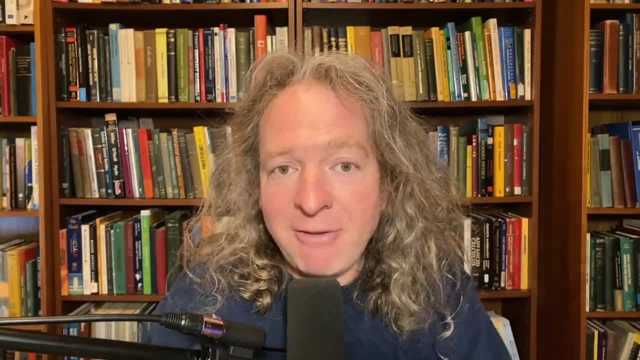 so assuming you don't know how to write proofs that's what you do after that what do you do what's your path then that's when the world opens and the world is yours in the world of 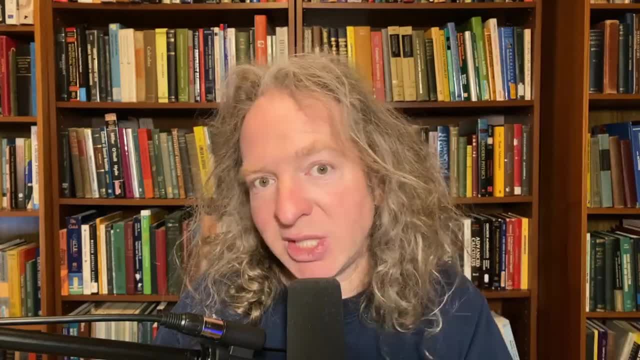 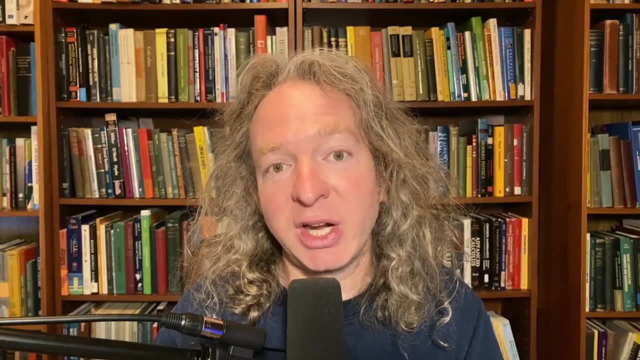 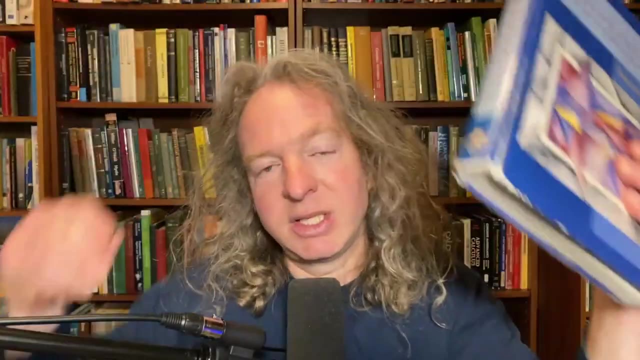 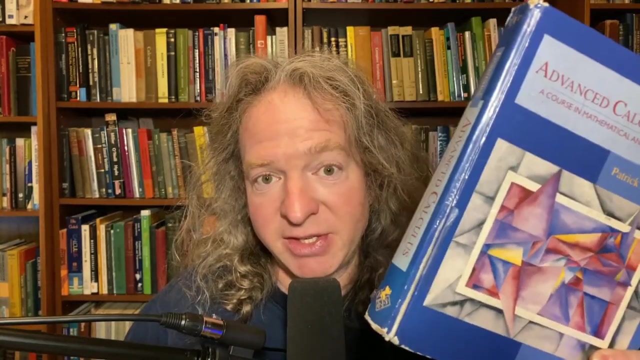 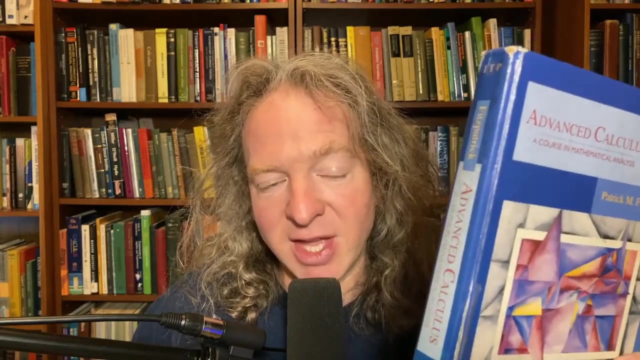 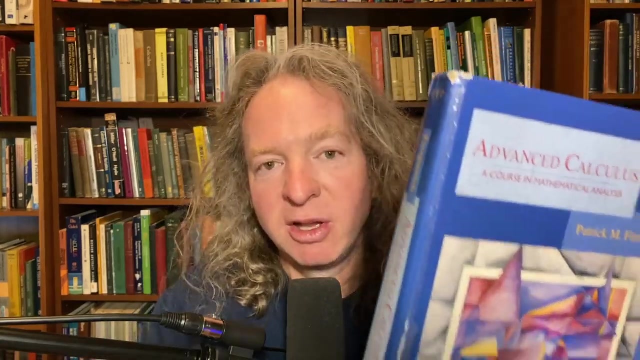 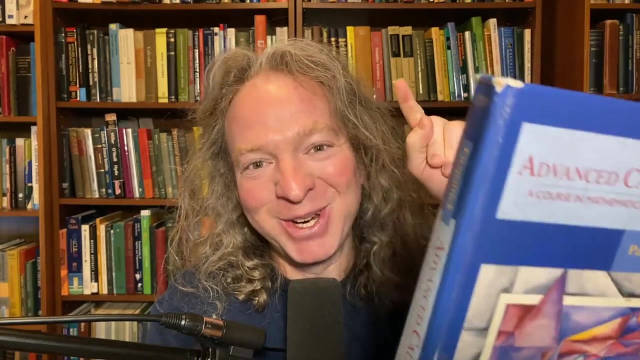 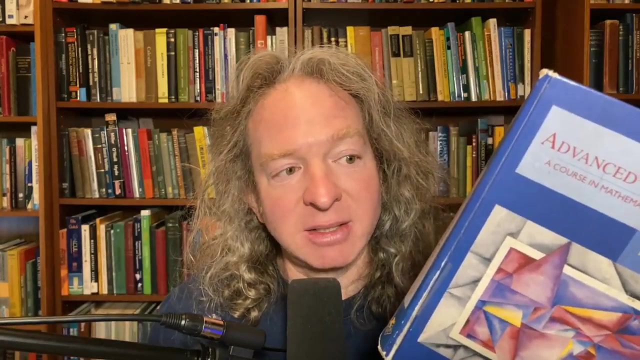 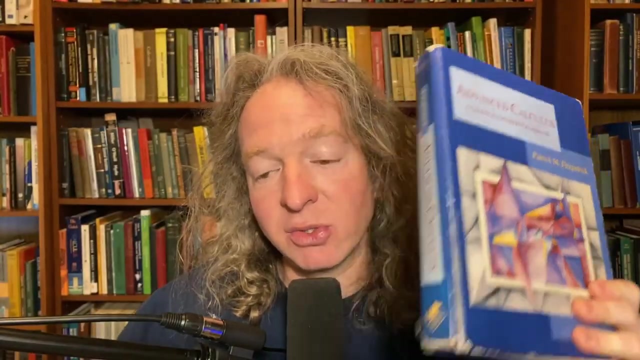 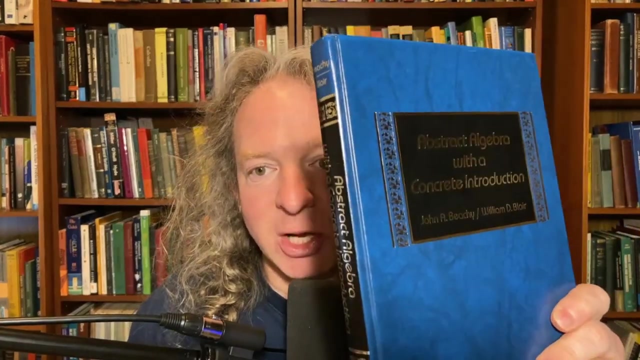 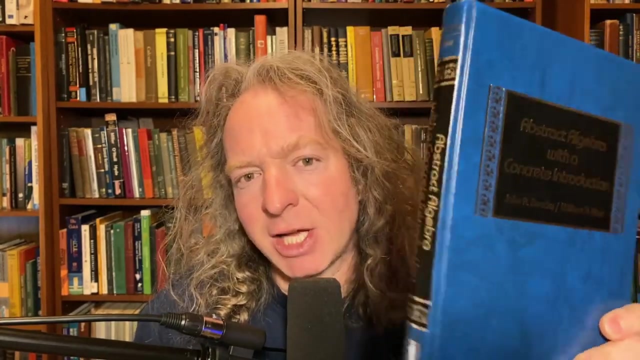 mathematics because once you know how to write proofs you can really take it to the next level and again it's a slow process it's gonna take persistence and time but you're really gonna learn a lot of mathematics so like let's say you know how to write proofs then what you do is you get a book like this one this is advanced calculus a course in mathematical analysis by fitzpatrick you know you can get this book you used um this is this is the first real analysis book i use that's why i wanted to show you this one so i've read good portions of the book i've done a ton of the exercises it is hard you're gonna think this is not a very good book you're gonna you're gonna buy this book after you learn to write proofs you're gonna sit down with it and you're gonna struggle and you're gonna have a hard time it's one of the easiest books so there's there's worse right there's books out there that are so much harder than this one so it's hard it takes time and yeah that's my answer so start with proof writing and then you can move up to books like this if you want to learn advanced calculus or or say you want to learn something like abstract algebra another book I'd recommend would be this one here abstract algebra with a concrete introduction by Beachy and Blair I believe the new one is just called abstract algebra so you can just get abstract algebra by Beachy and Blair fancy cover here right really pretty book but those 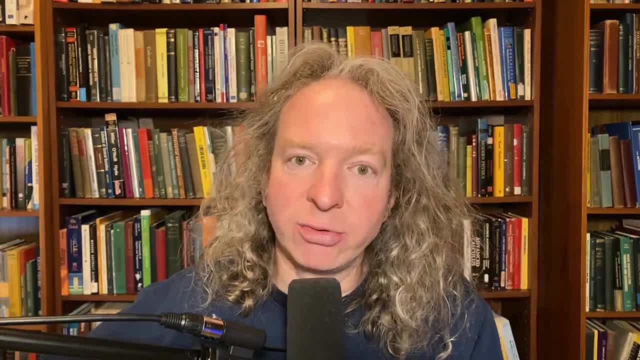 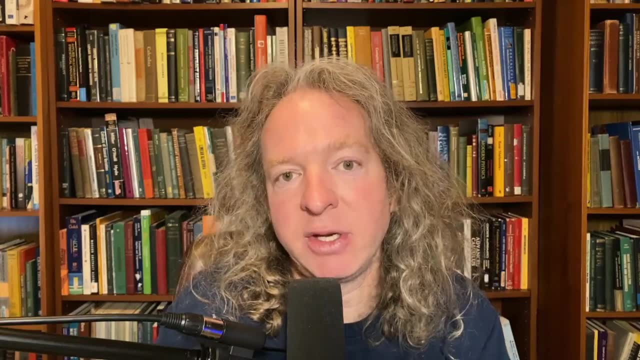 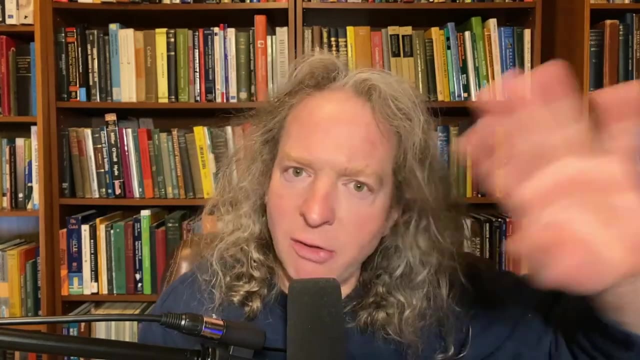 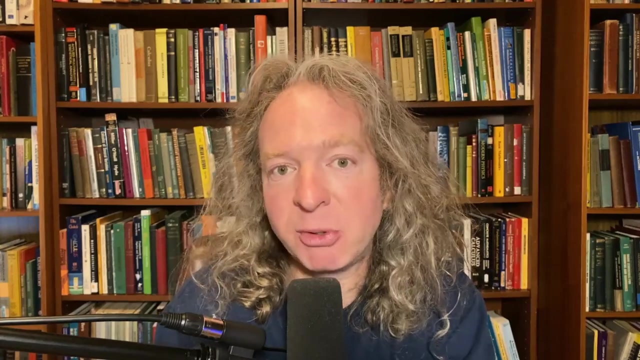 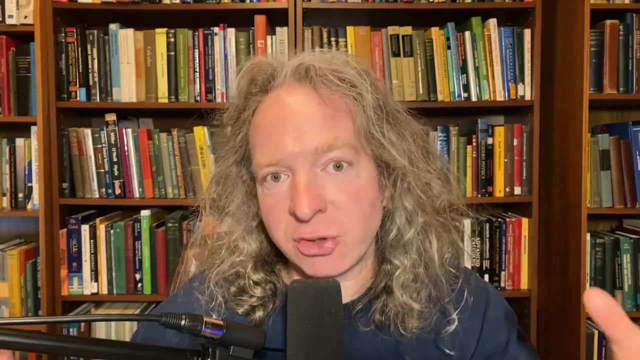 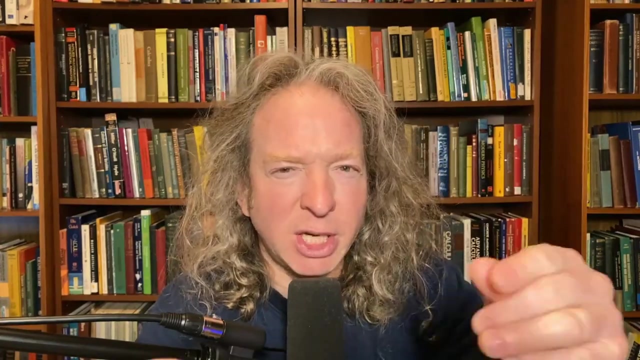 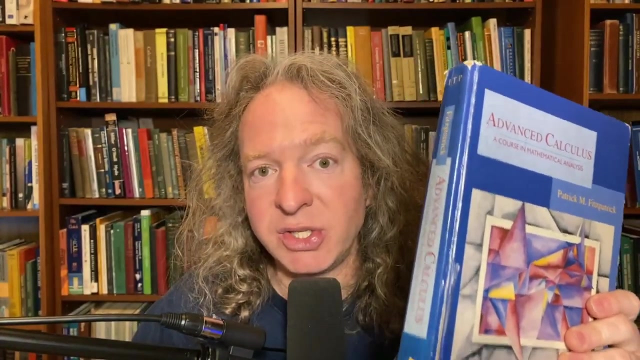 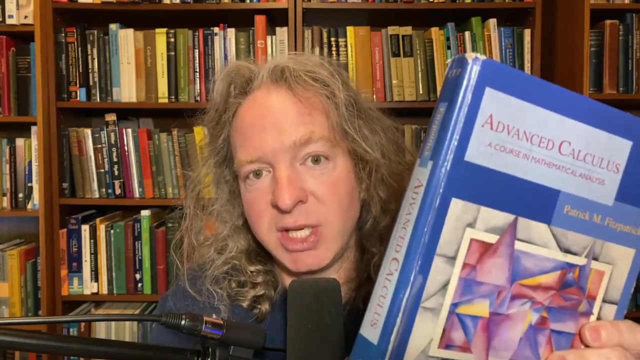 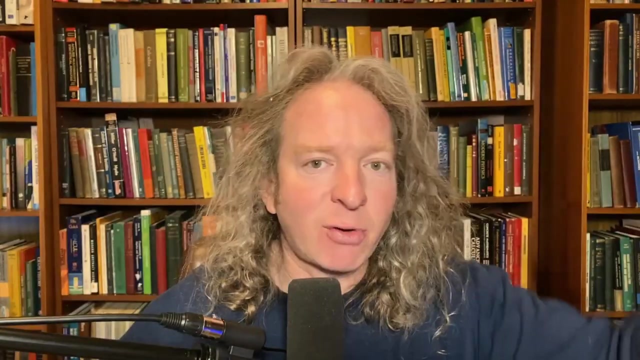 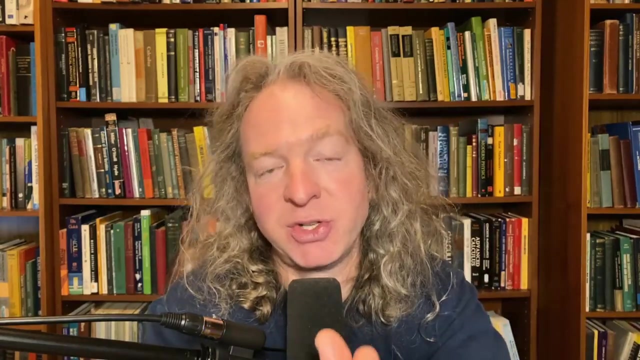 are the ones that are really good at advanced calculus but you can't really do that until you get the proof right so that's going to take you to the next level because I'm pretty sure that like most of the videos like most of the math videos that are on YouTube and are popular like like mind your decisions and like those other channels and all the math videos if you watch a math video on YouTube typically typically it's not a proof right because people don't most people don't know how to write proofs right so if you're watching math videos for fun typically it's something that like most people understand like an integral or equation something that like is tricky and interesting that's typically what you see on YouTube in terms of math videos tricky interesting problems that are accessible to most people whereas the problems you're going to be doing in here are serious heavy you know theory based proof based mathematics which take a lot of work and you don't you do see these you do see examples like the ones in this book on YouTube like I have videos um you know from from problems in this book and abstract algebra I have a whole abstract algebra playlist a whole advanced calculus playlist on YouTube but it's you know it's not that tight it's proof-based right so you're going to get proofs so you can do that too you can watch 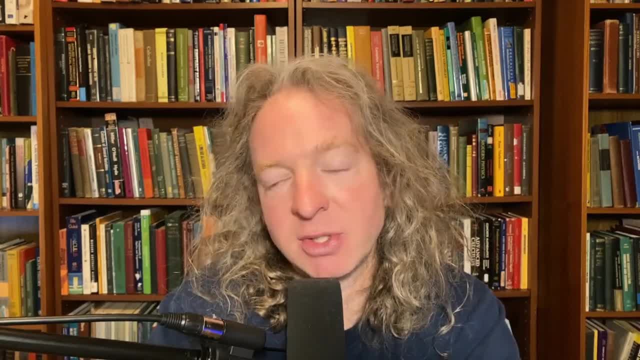 videos like that and there's other channels that have proof-based videos and that's really what's 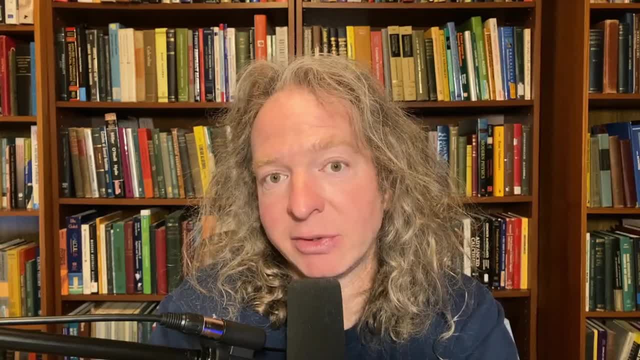 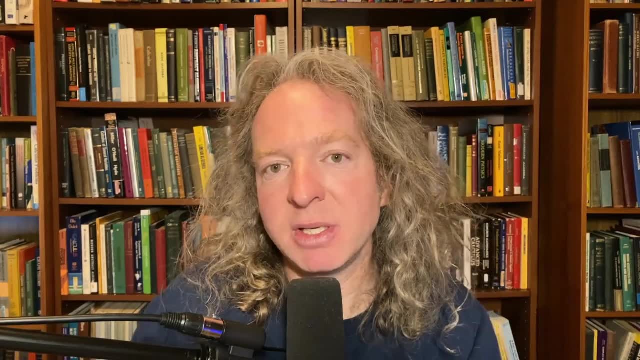 going to help you um take your math to the next level so yeah 30 minutes a day learn to write proofs and go from there and another reason I say learn to write proofs is because a lot of people 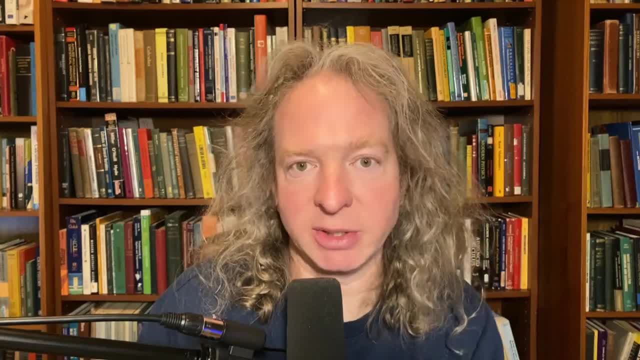 um when they first see like calculus 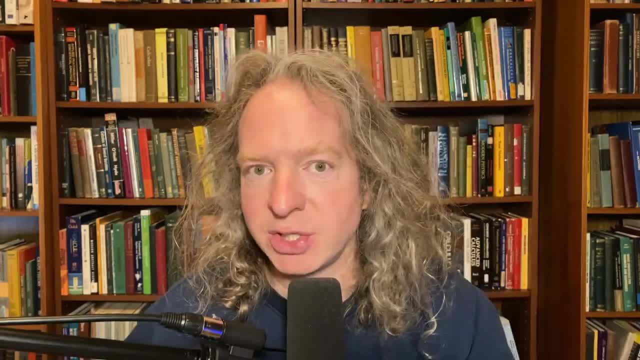 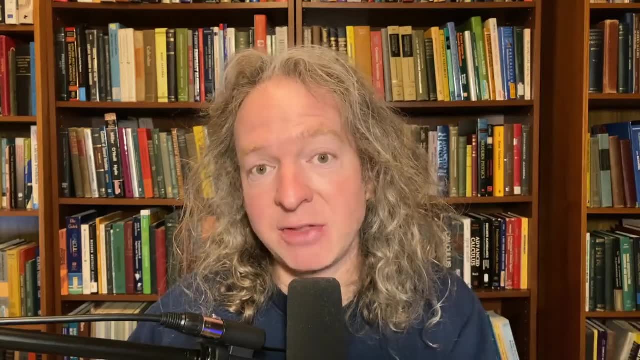 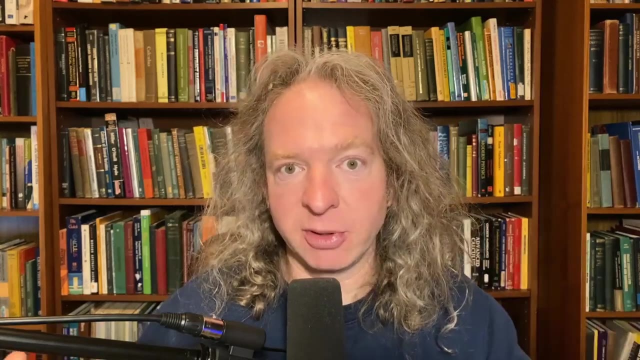 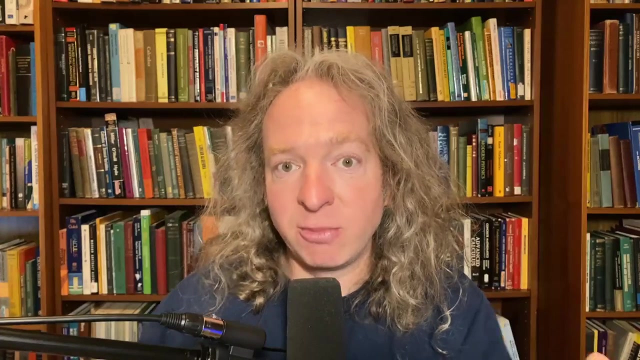 they say oh I really love doing integrals I love integration oh I love integration by parts you know and that's great you should be excited about it but that's not what all math is like math changes there's different types of math and proof proof is key proof is beautiful I'm getting goosebumps mathematics is about proof and discovery right so it's about discovering new mathematics and then proving those things that's that's one way to look at it a simplistic way to say what mathematics is right proof and discovery 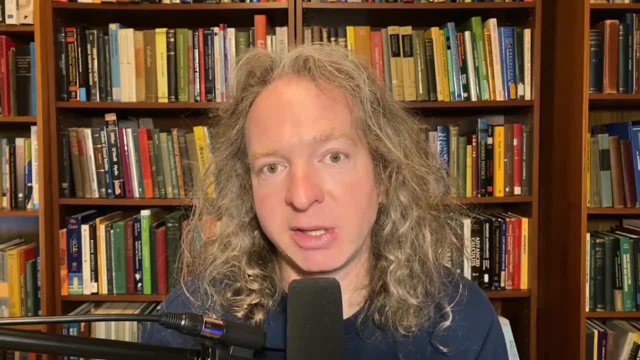 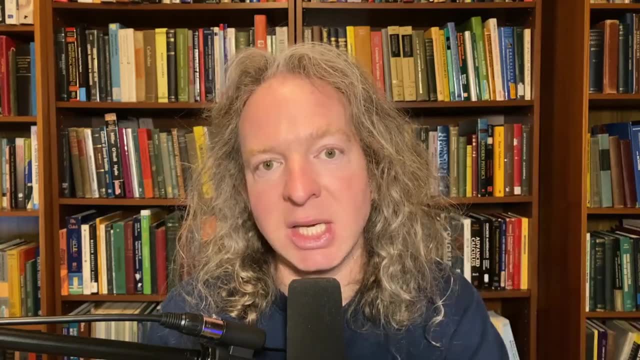 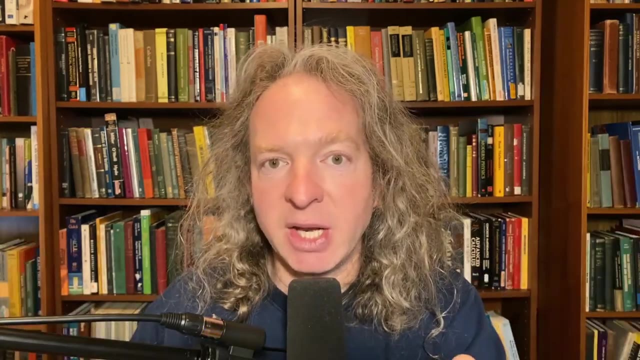 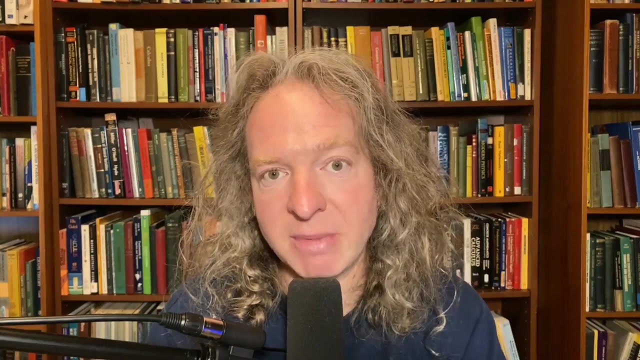 discovery. And the proof part is the part that typically only math majors learn or computer science majors if they take a course called discrete math. And that unlocks the key to take you to the higher level math. Again, once you know how to write proofs, you can learn most of the stuff I talked about in everything actually in that learn math from start to finish video. You can learn everything. If you go to college and you get a four-year degree in mathematics, what do you 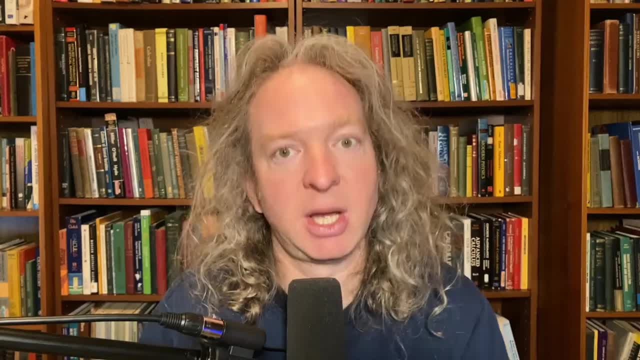 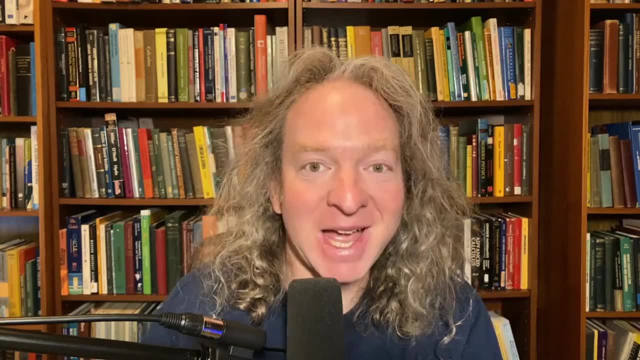 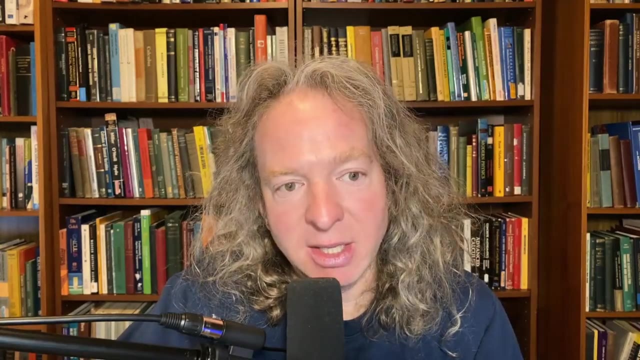 come out with? A lot of knowledge and the ability to write hopefully decent proofs. So start with that and then go from there. If anyone else has any advice, please leave a comment in the comment section below. People do read the comments and I think it helps other people. Again, this person's 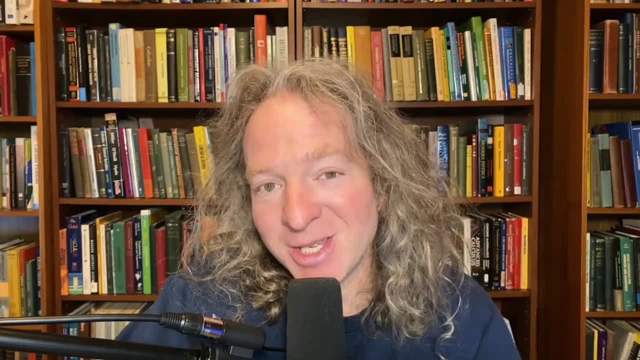 name was Jovan and the question was advice for medical students. Speaking of medical students, 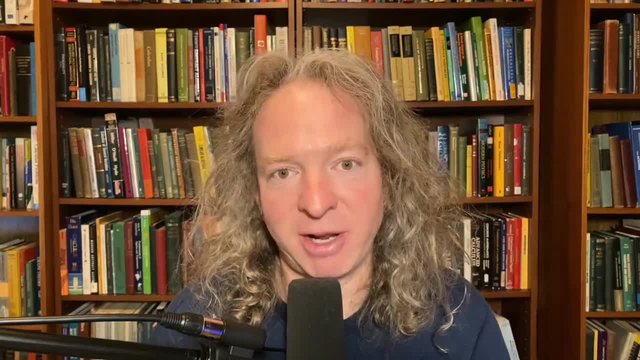 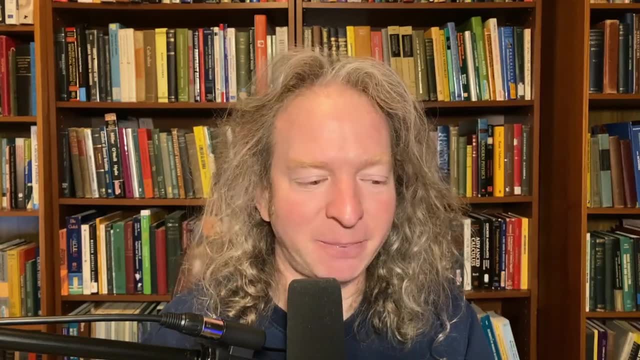 it's funny. I have a story. Now, this is not my story, but I'll finish the video with the story because I think it's an interesting story. I think it's an interesting story. I think it's an interesting story. So why not? I'll share it. I got time. I was reading a book. It was a book 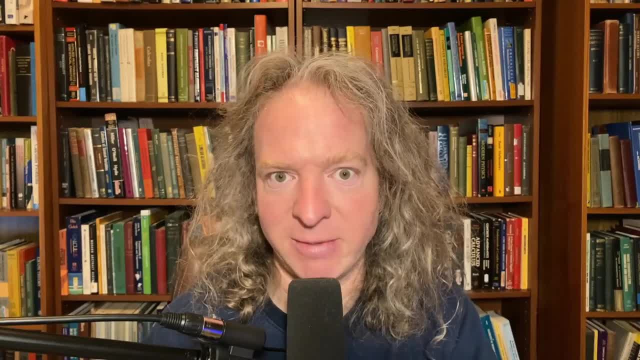 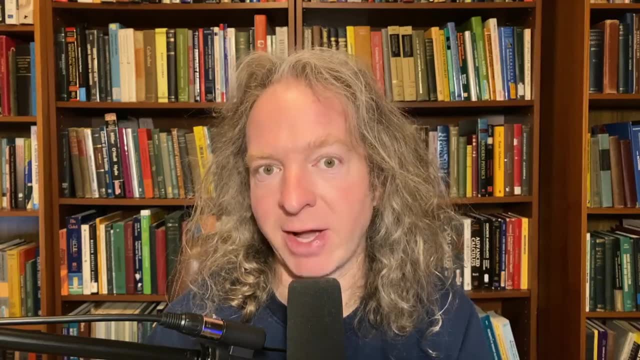 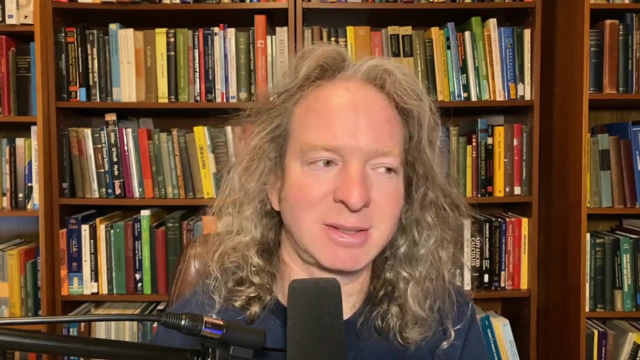 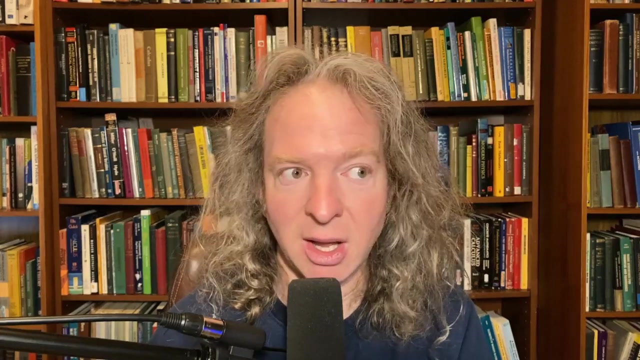 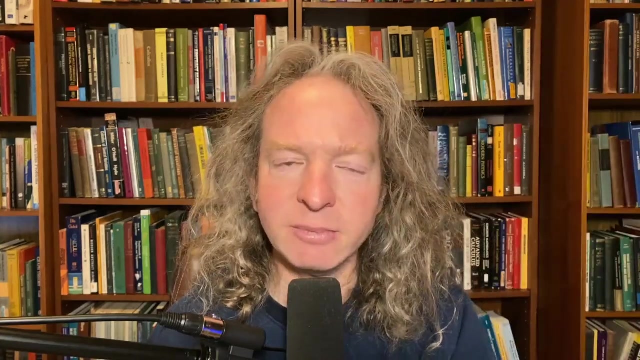 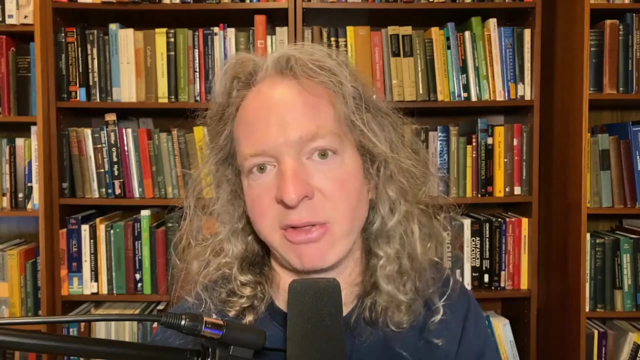 written by a mathematician who's I believe still alive and very famous. His name is Stephen Krantz and he has a book. It's called A Mathematician's Survival Guide. I did a review of this book long ago. I think it's been like three years and it's probably like it's probably the most useful book that a person who is interested in a career in mathematics should purchase. Okay. I've read the entire book multiple times. I've read certain chapters like three times. I adored the book when I was an undergrad. After teaching and getting some actual like life on the job experience, teaching at a college for several years and seeing how things work and, you know, just seeing the psychology of it all, you know, what's expected from the math department. What 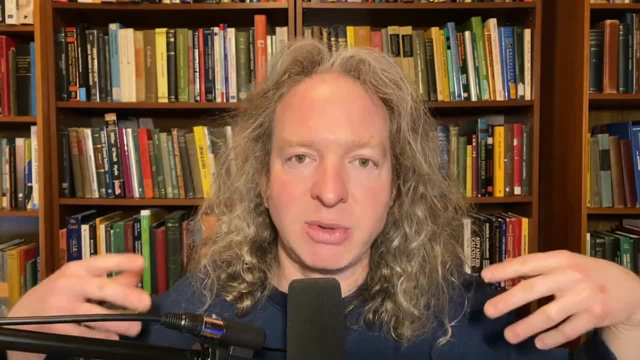 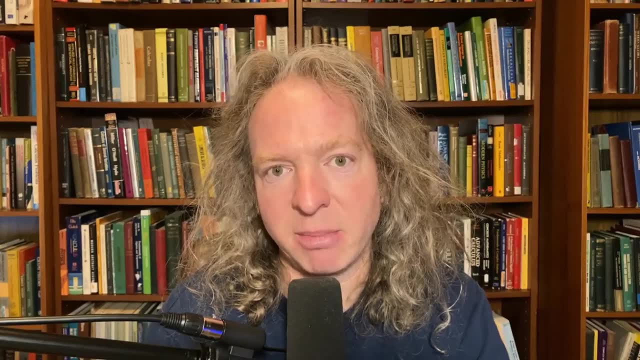 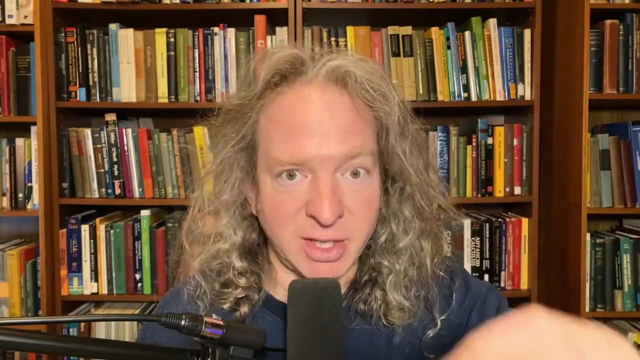 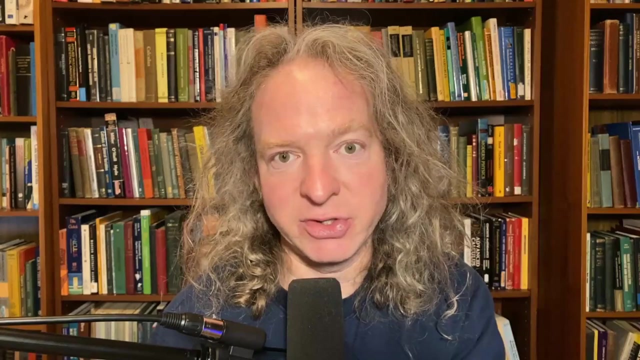 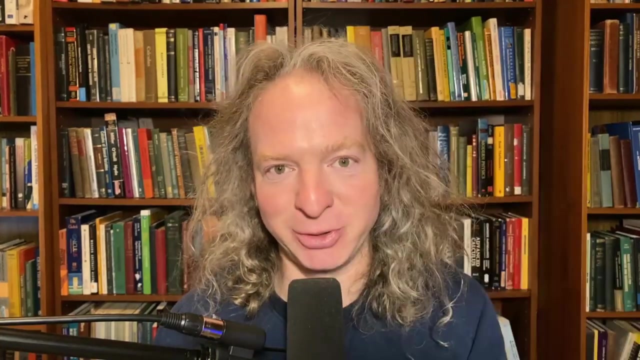 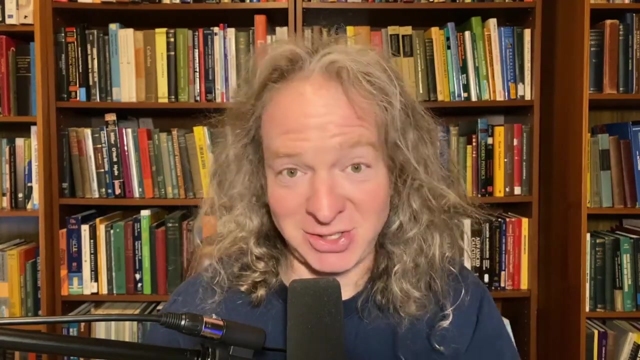 do the students expect? You know, all kinds of stuff you learn about teaching when you actually deal with people in your teaching. And I realized that the book is not perfect. I don't agree with everything Krantz says in that book. But in the end, it's a book that I'm going to read. And I think in that book, you will learn what it's like to, you know, to be, you know, a math person, like to be a teacher, to be a TA in grad school. It explains everything. Anyways, I digressed. He talks about how at his university, I believe it's Washington University at St. Louis. And this is from the book. And I'm paraphrasing. There was a person who was a medical student and he wanted to get a PhD. And he's like, hey, can you let me in? I want to get a PhD in math. This is the story. And again, I'm paraphrasing. 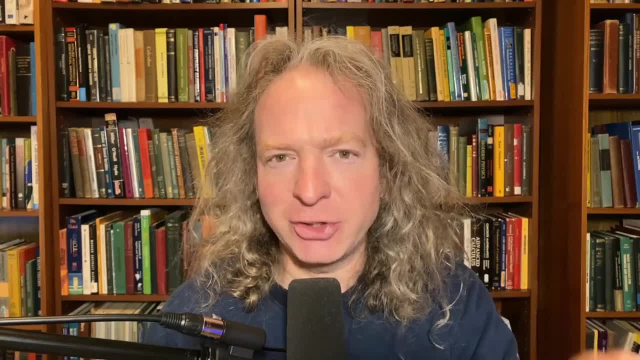 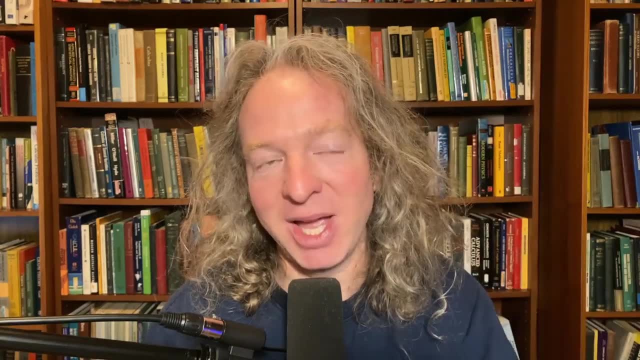 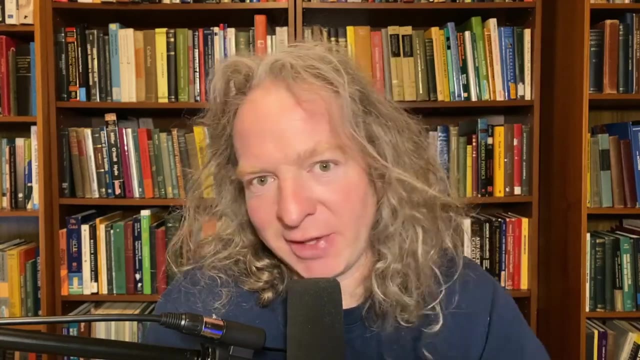 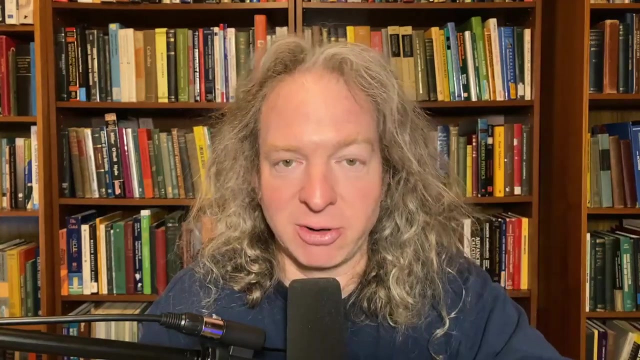 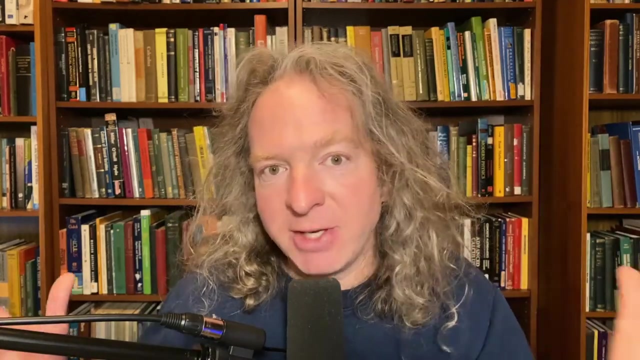 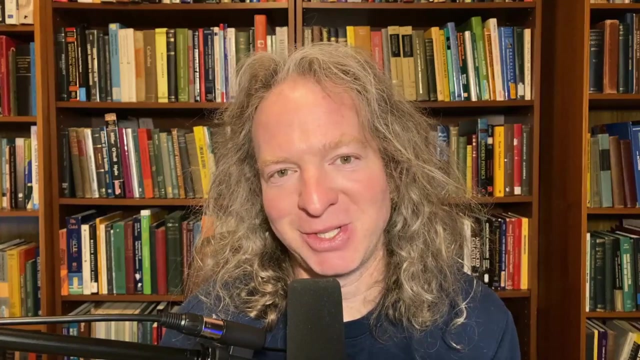 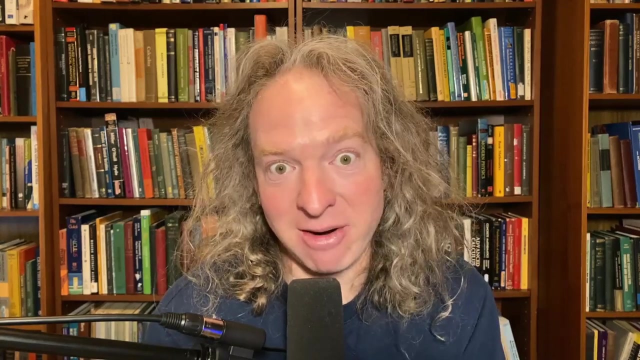 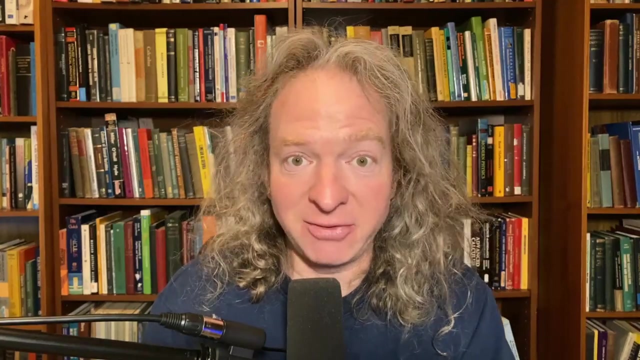 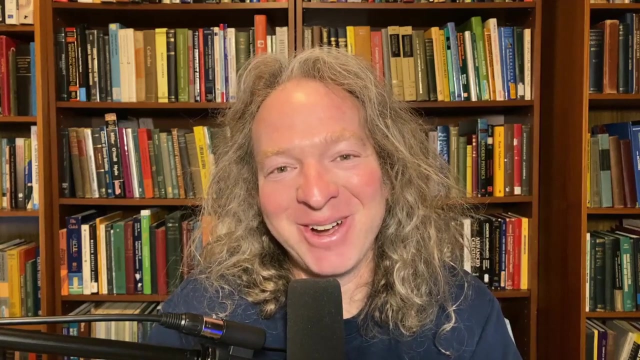 And he said, okay, we'll let you in. And he, I think he chose to like pay his own way. Like that's expensive, right? Grad school's not cheap. Usually it's free. So it's not cheap. So he paid his own way. And I think the story goes something like after a few months or a few weeks, he was like, this is so hard. This is so much harder than med school. And then like, I think he didn't finish because it was just incredibly hard compared to med school, right? PhD in math is so much harder, according to this one guy. So fun story, right? About a med school student going back. And I don't know what happened. I don't know if he got his PhD or he quit. I don't remember the story. The story is, it's in the book, A Mathematician's Survival Guide by Stephen Kranz. So you're not the only med student to want to go back to school and study math. But I think that's hardcore. Medicine is hard, right? I mean, the fact you're in medical school, that is no joke, right? To get into medical school, at least in the US, it is very difficult. It's, you know, you're going to be a doctor. So it's a really good thing. Anyways, kind of a long video. 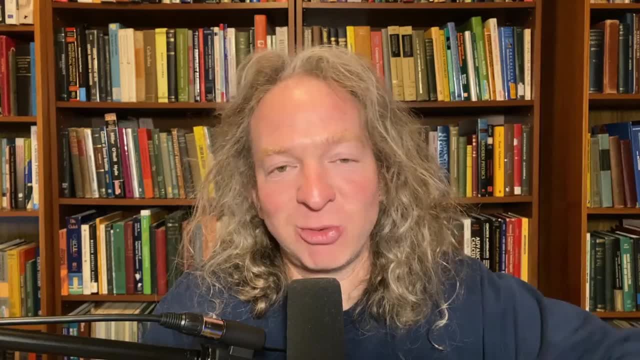 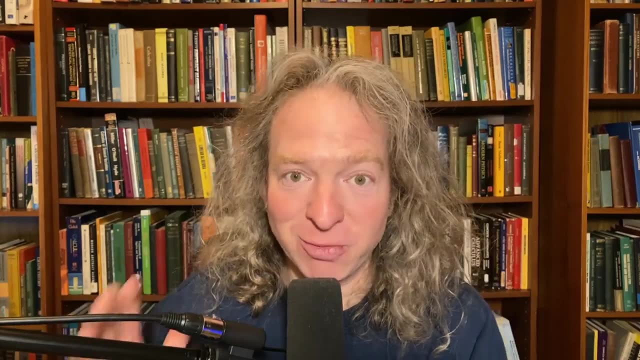 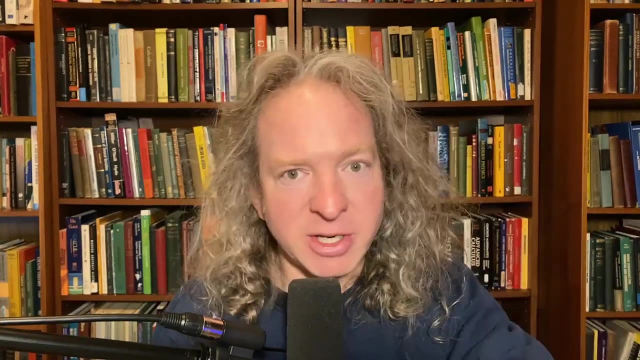 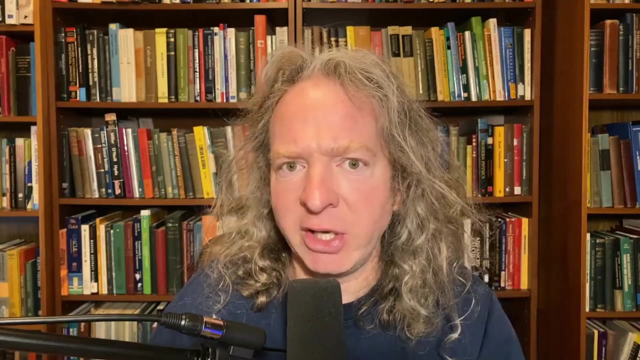 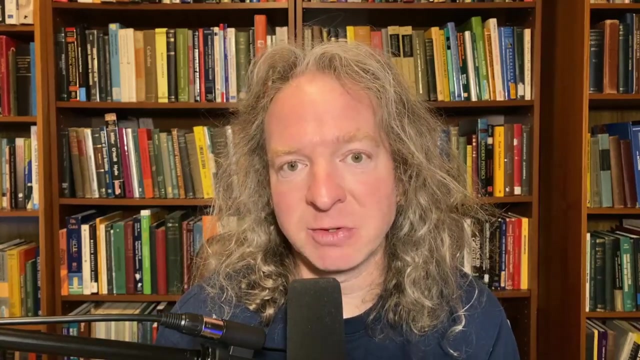 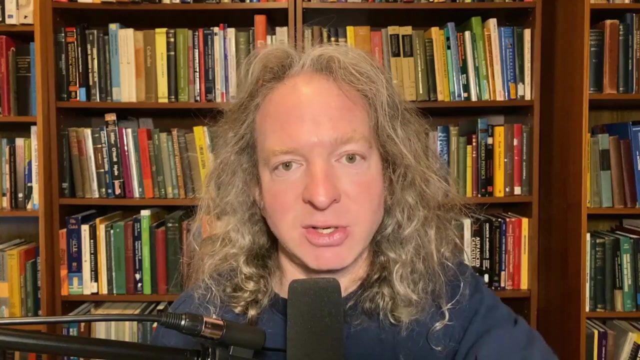 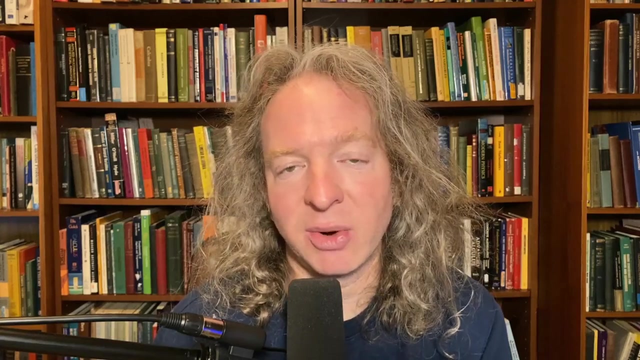 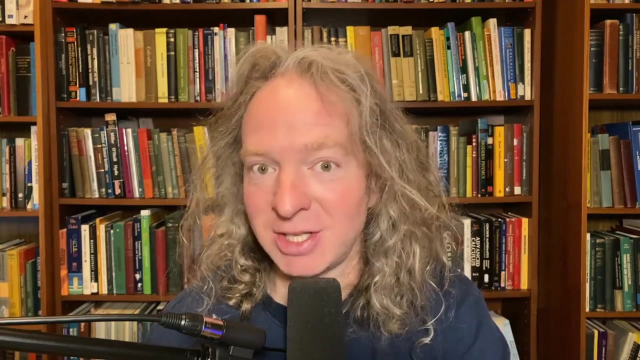 And hopefully this has helped someone else out there who's watching this on YouTube or listening via YouTube's new podcast thing or Spotify. But yeah, that's my advice. Start with proofs, right? Start with proofs. That's really going to open the door. And that's the advice for anyone who is thinking, oh, I want to get, I want to really learn math. If you already know some math, start with proofs. If you don't know any math and like your math is really, really bad, learn some algebra and stuff first. Get familiar with the lingo. Get some exposure to like trying to read math books. It's a real struggle when you're learning. And then jump into proofs. But the book by Vellman, beautiful book. I recommend it. I'll try to leave a link in the description of this YouTube video. If you're watching this on YouTube, you can see it there. And book of proof, it's also free. You can just Google that, but I'll leave a link as well in case you want to check that out. Anyways, until next time, thanks for watching. And if you're watching this on YouTube and you're still watching this, if you've made it this far in the video, oh wow, this is a 14 minute video. 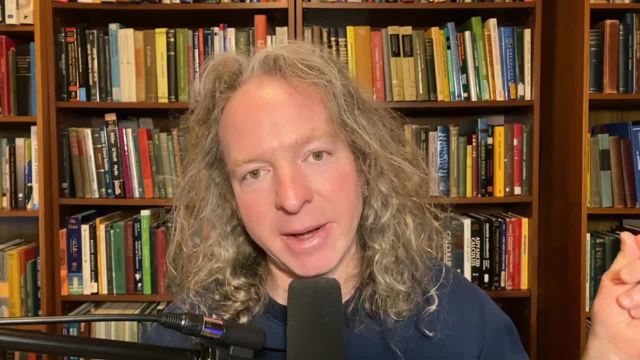 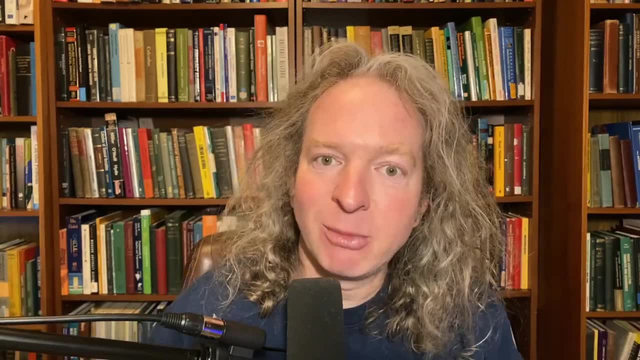 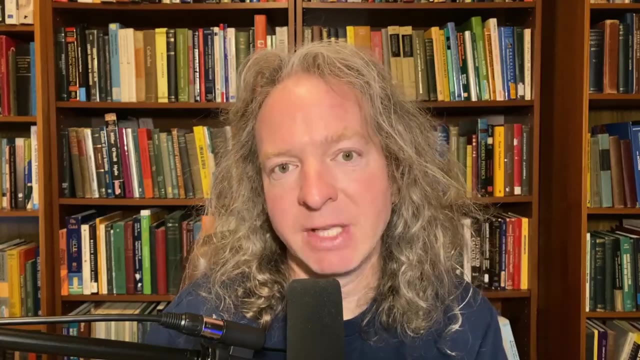 Make sure to subscribe, right? Subscribe to my channel. I usually, post videos like this. This is for my podcast. I also post other videos. This one is 100% unedited. I just had my morning coffee and I wanted to reply to an email, at least one email here on the channel. So yeah, good luck. Take care. Keep doing math.